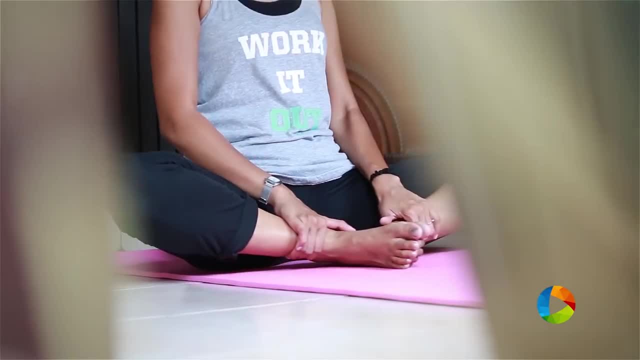 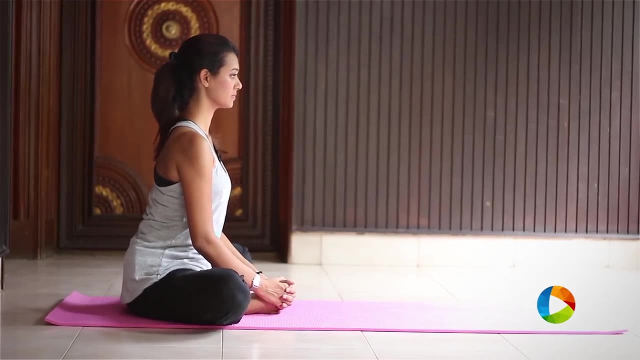 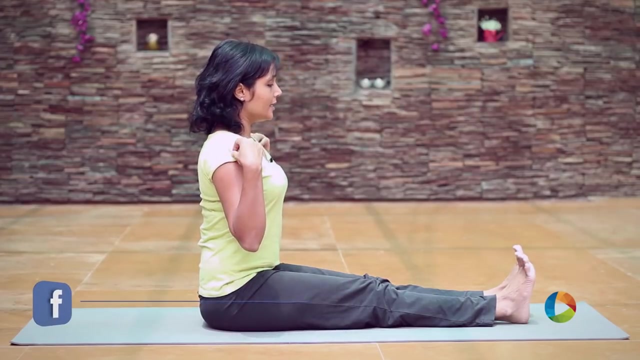 the stretch in your groins. pull your feet closer to your pelvis and begin to flap for a couple of times. Bring both your legs out in front of you, pointing the toes inwards. See to that your back is straight and the spine is extended, with the chest opening giving. 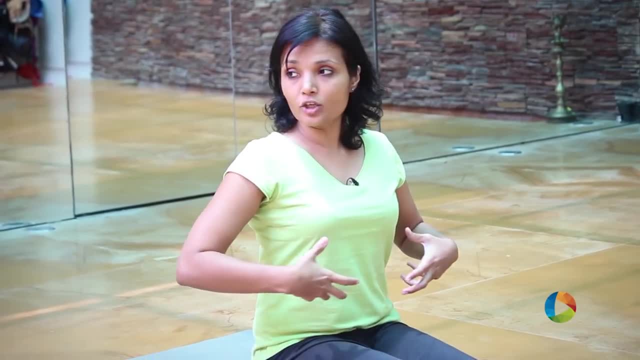 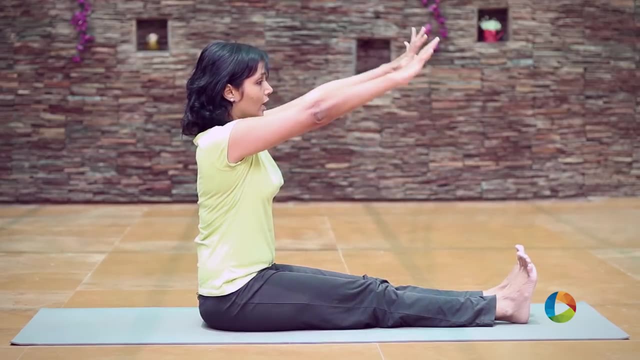 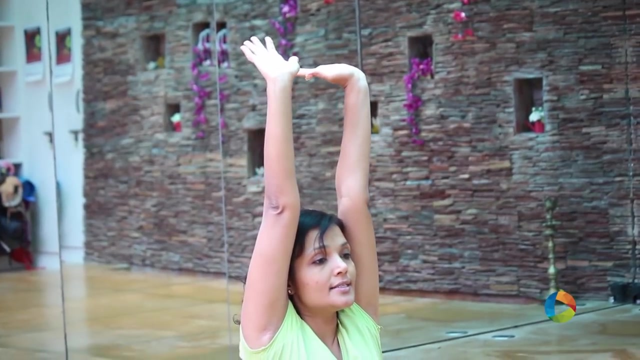 your body and your lungs enough space to breathe. The ribcage should have enough space for your lungs to be able to expand. As you inhale, you raise both the arms up, extending the spine further, bringing the hands in line with the ears. As you exhale, you bring the chin out and come down as low. 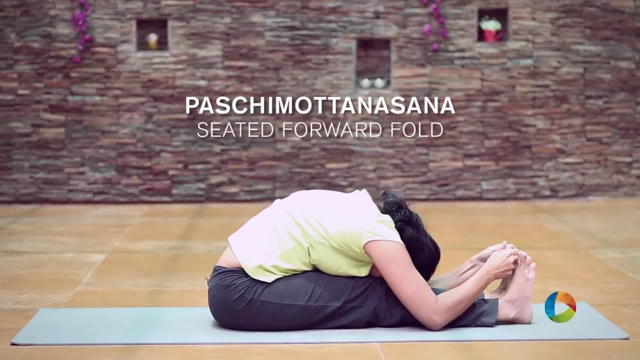 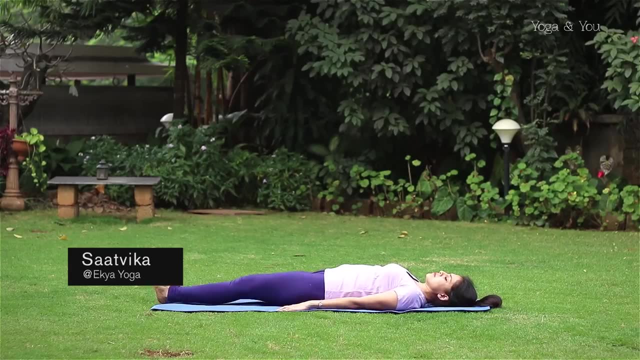 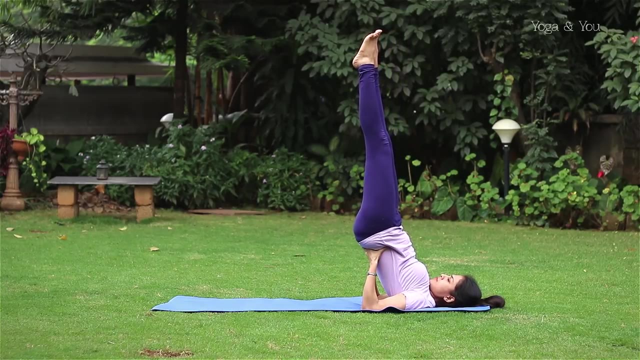 as you can. If you can, you hold your toes, bringing your forehead to rest on your legs. Raise your legs, lift your hips up and support your back. Stay there for a few breaths To adjust. bend your knees towards the forehead, tuck. 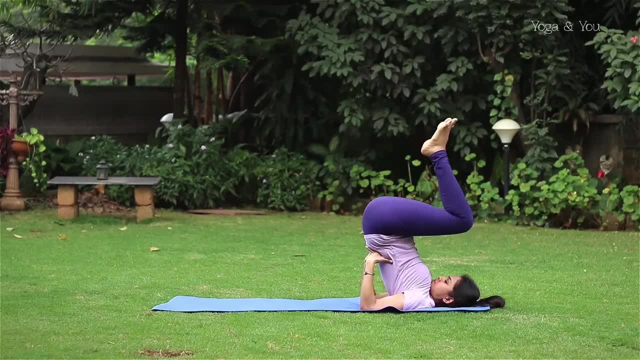 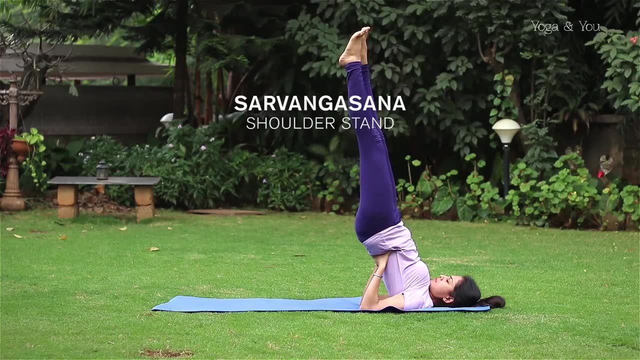 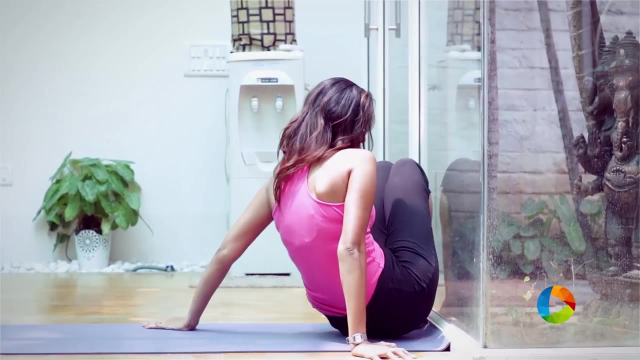 your elbows in closer together, walk your hands down your back and then straighten the legs So you want to come closer to your wall and place your butt as close as possible. Just begin to lie down comfortably and place both your legs all the way. 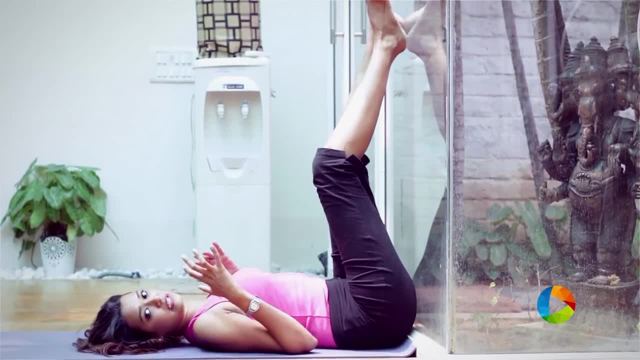 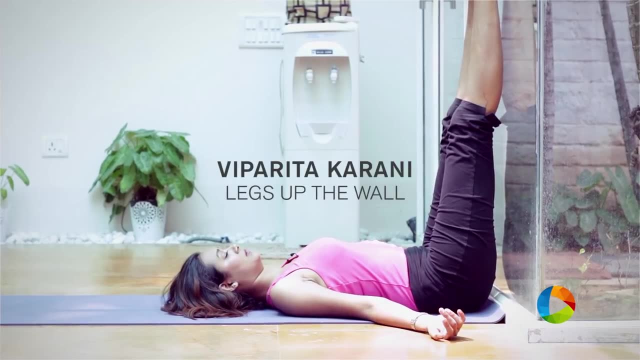 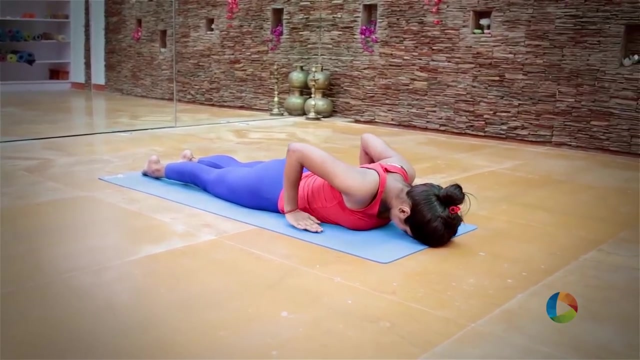 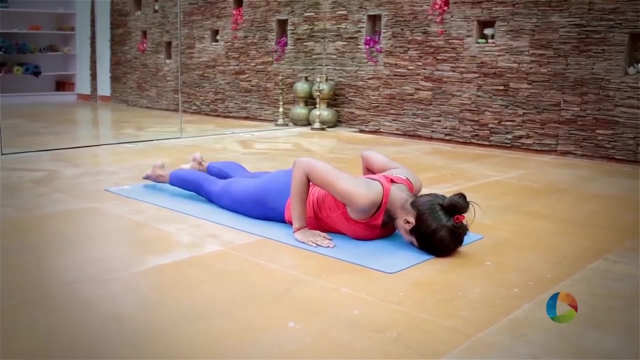 Lift up and still just scoot yourself closer to your wall. See, my butt is as close as possible and relax. Now gently place your hands down in between your shoulders and your pelvic bone, Open your legs slightly out, Inhale and then come up. Now lift your hips up and come down. 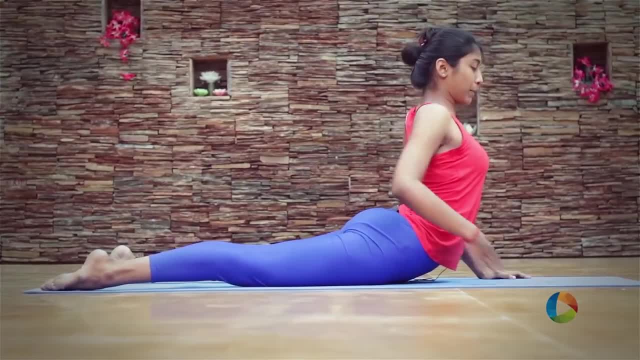 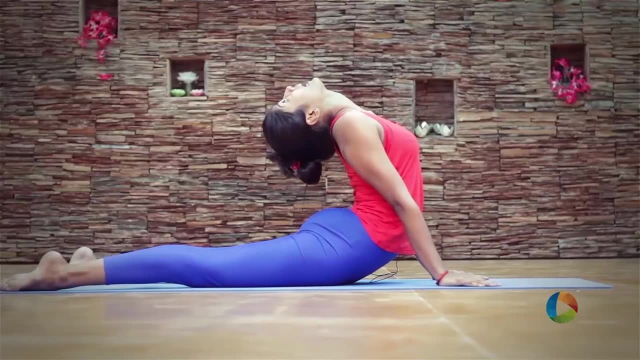 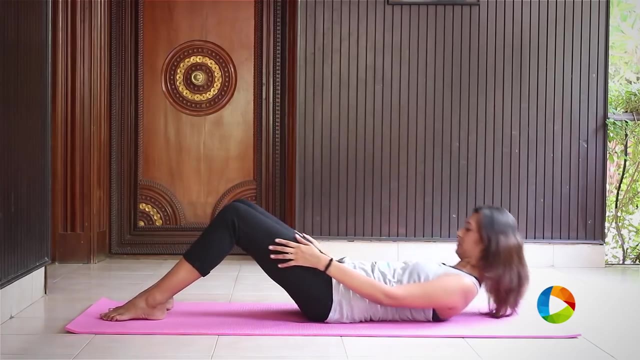 Lift your navel above the ground level. Push your pelvic bone down. Procure your pelvic bone down and then elbow straight, Push the shoulders back, draw them back to the heart, Begin to lie down on your back and place your heels as close as possible to your butt and